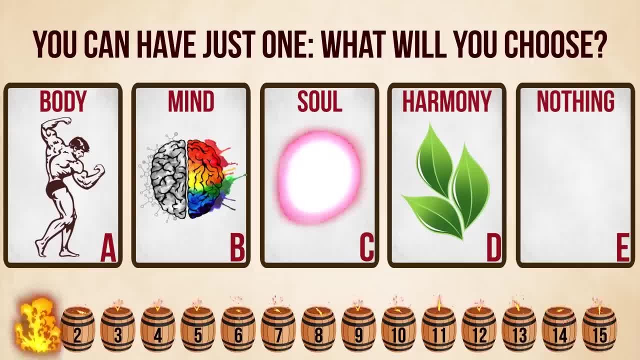 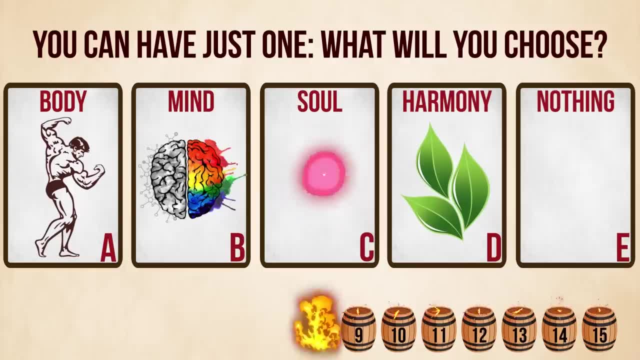 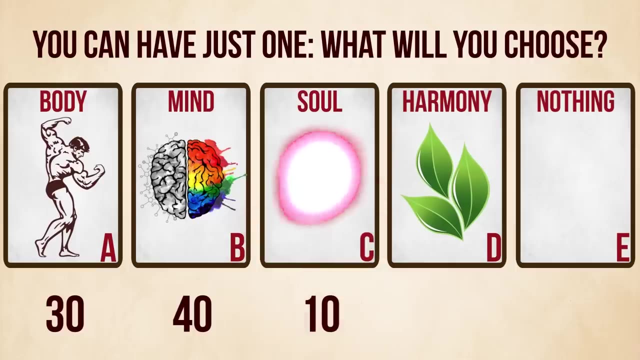 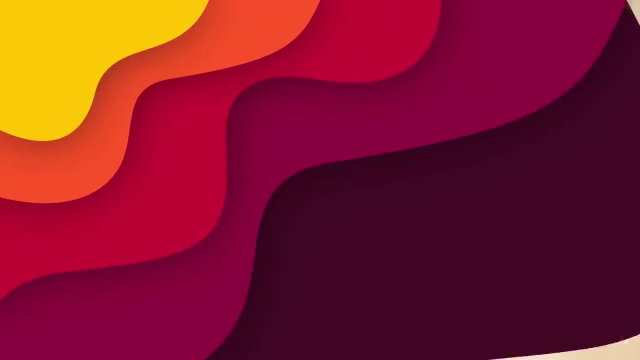 Nothing Score. Answer A gives you 30 points, B is worth 40 points, C is 10,, D will be 20, and option E will award you a whopping 50 points. You get 50 points. Question number three: 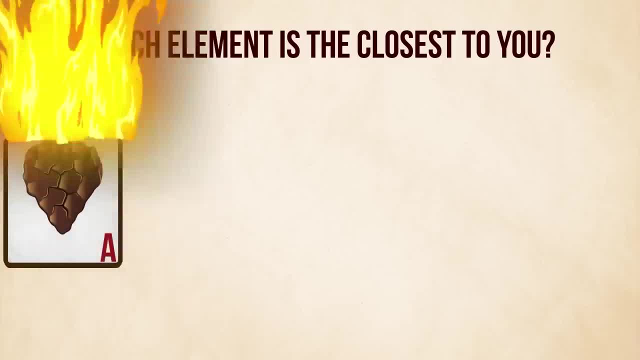 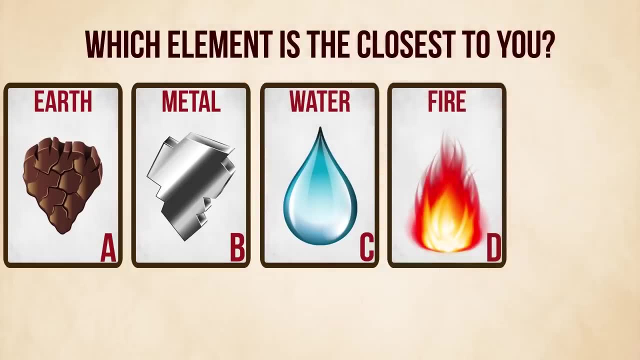 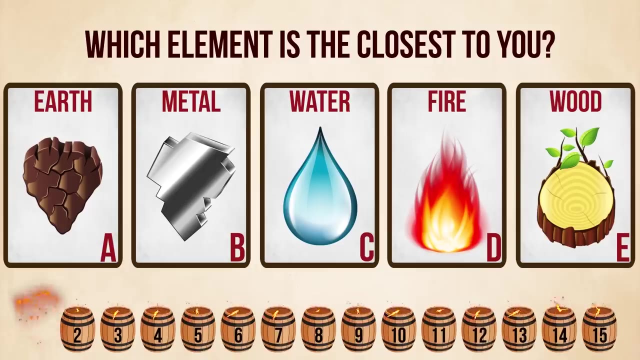 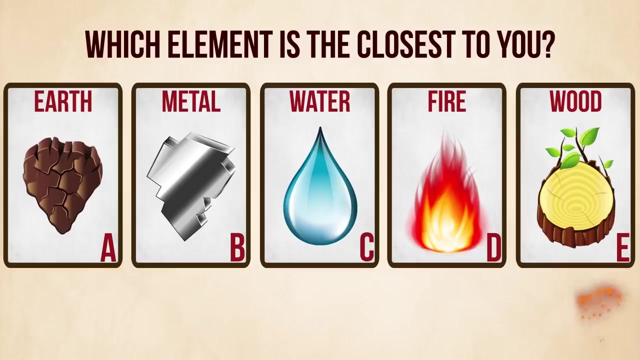 Which element is the closest to you? A- Earth, B Metal, C. Water, D Fire, E. Wood Mod massage sounds. Concern Valley, Arizona. C&O Farms. Score: Earth lovers get 40 points for choosing A. 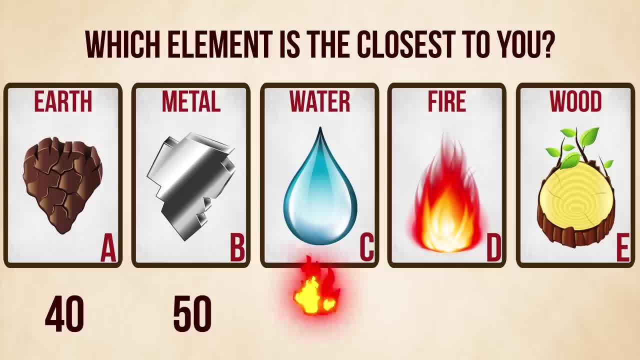 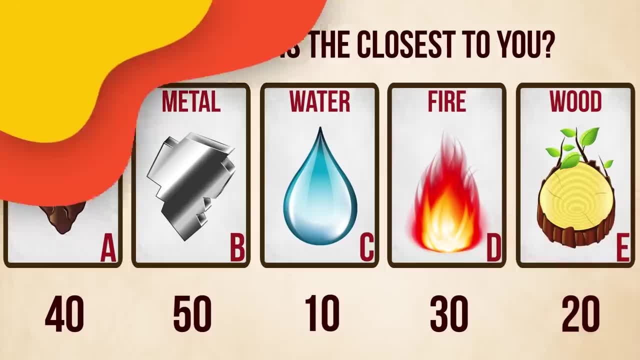 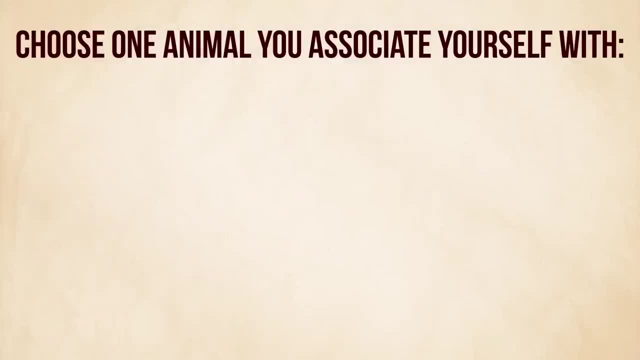 As for B, it'll give you 50 points. Add 10 points to your tally if you chose C or 30 if you went for D. Answer E will bring you 20 points for this question. Question number four: Choose one animal you associate yourself with. 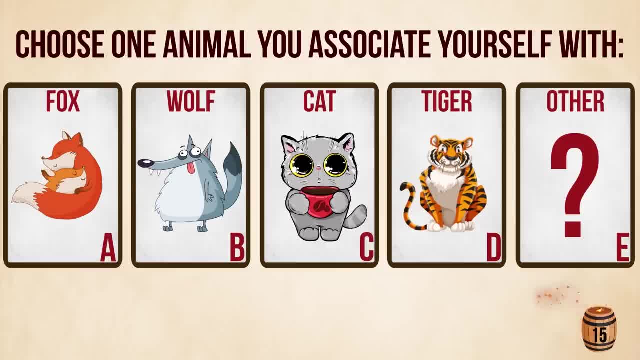 Answer E will bring you 20 points for this question Score. If you opted for A, you now have 40 more points. Answer B equals 10 points and C is 50 points. If your answer is D, that's another 30 points. 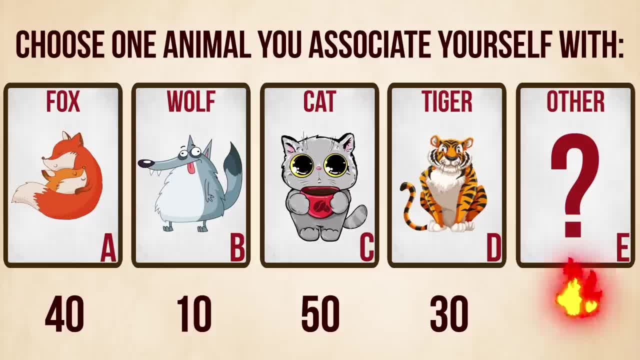 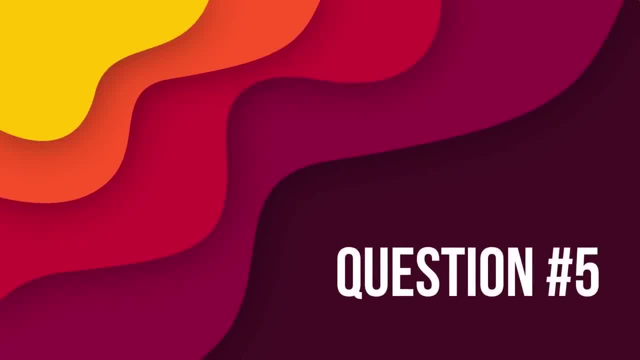 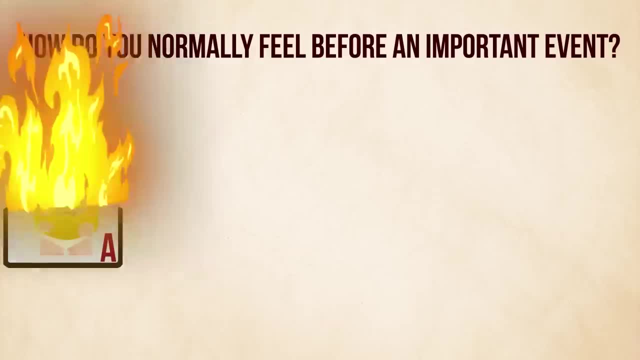 And if you aren't sure about your totem animal and chose E, give yourself another 20 points. Question number five: How do you normally feel before an important event? A- Anxious, B, Confident, C, Useless? 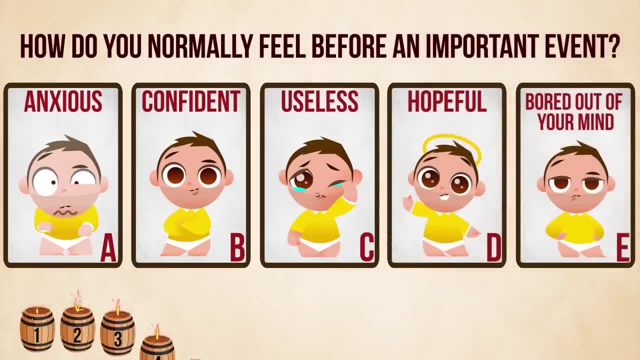 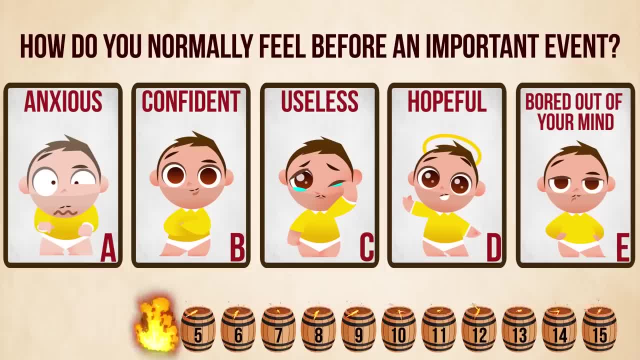 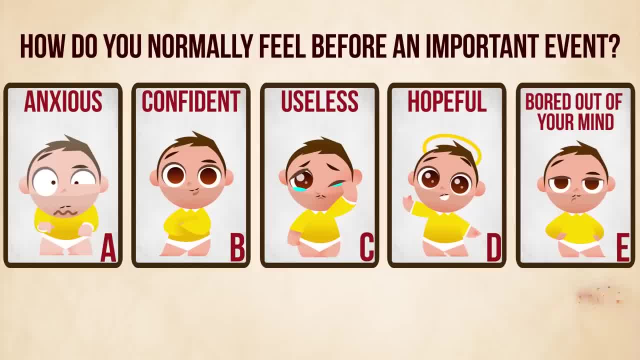 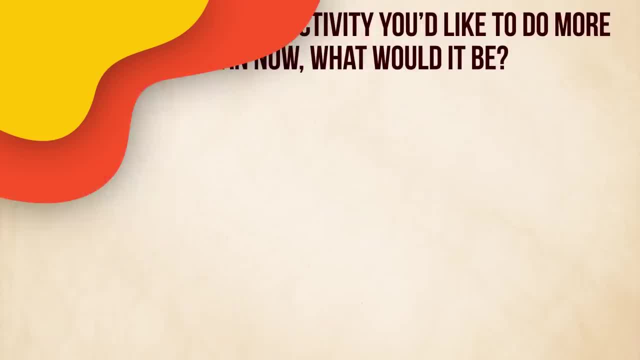 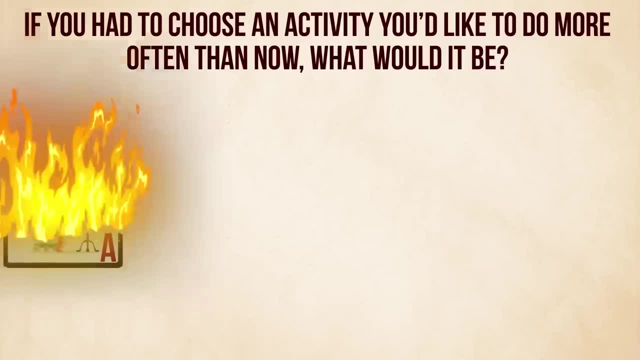 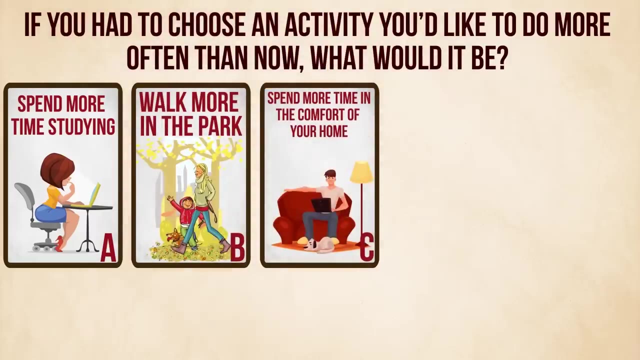 Question number six: If you had to choose an activity you'd like to do more often than now, what would it be? A- Spend more time studying. B. Walk more in the park. C- Spend more time in the comfort of your home. 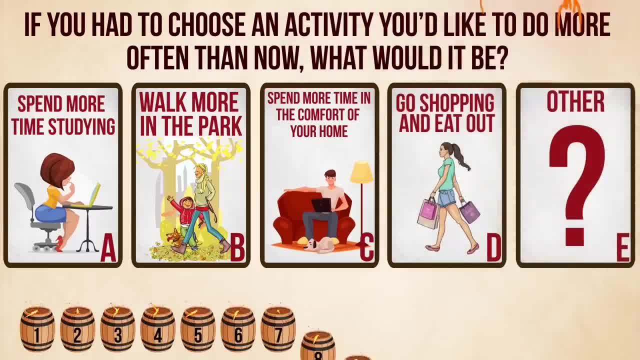 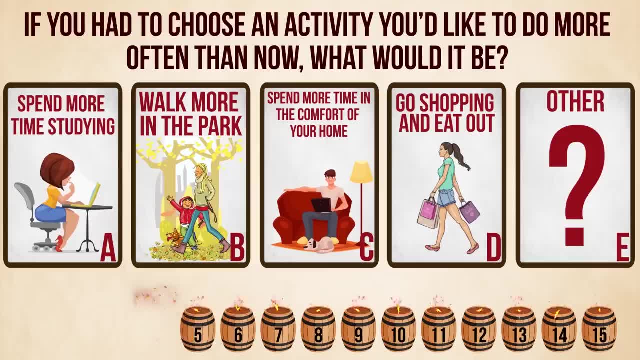 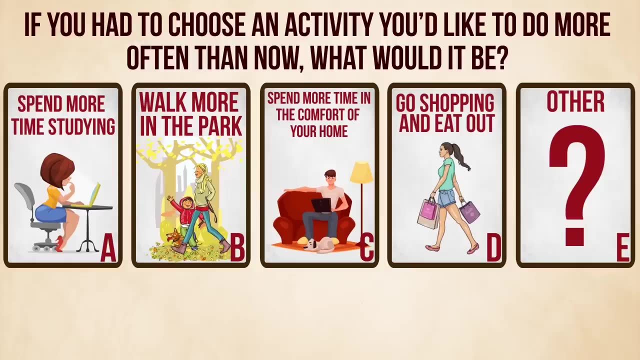 D- Go shopping and eat out. E- Other Score: If you just want to study more, give yourself 20 points for choosing A. As for those who went with B, you get 30 points. Homebodies can add 10 points to their tally for choosing C. 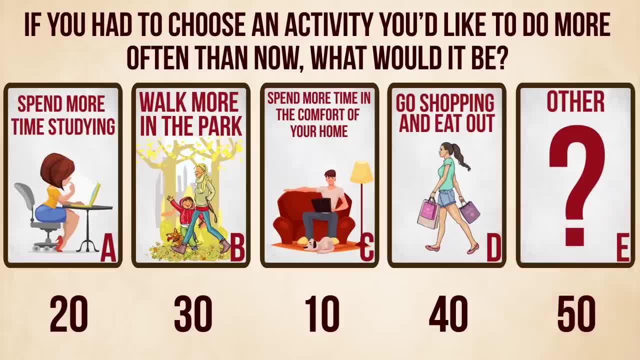 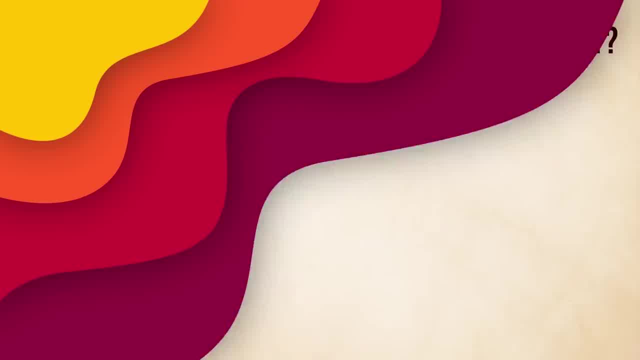 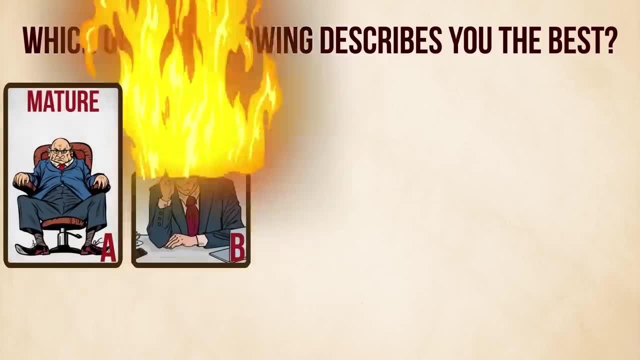 As for D, it'll give you 40 more points, and E is 50.. Question number 7.. Which of the following describes you the best? A, Mature, B, Brainy, C, Sensitive, D, Introvert. 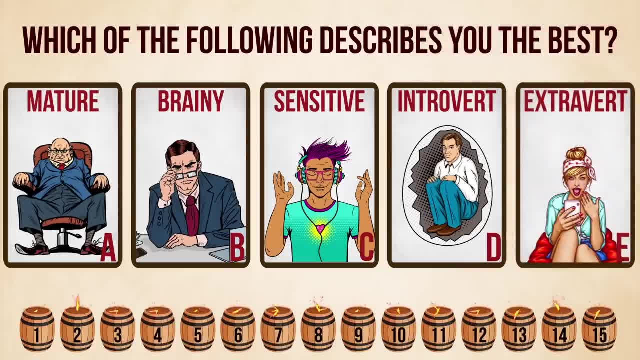 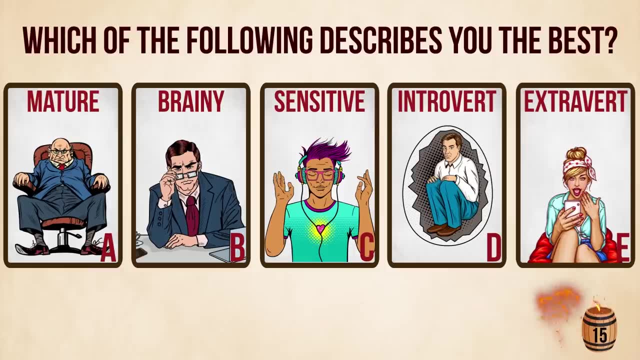 E- Extrovert: Score Your maturity for answer A will award you 10 points. As for the brainy folks who went for B, you get 30 points, C is worth 20, and D is 40.. As for you extroverts who chose E, you get 50 points. 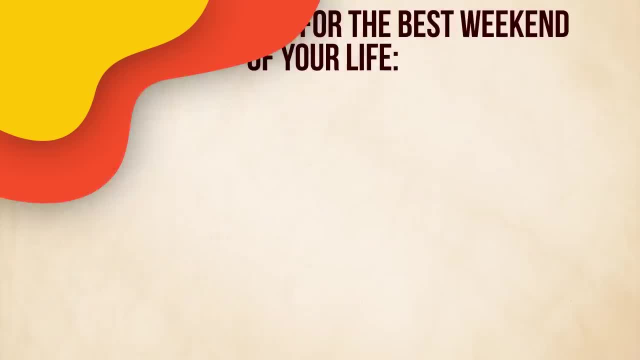 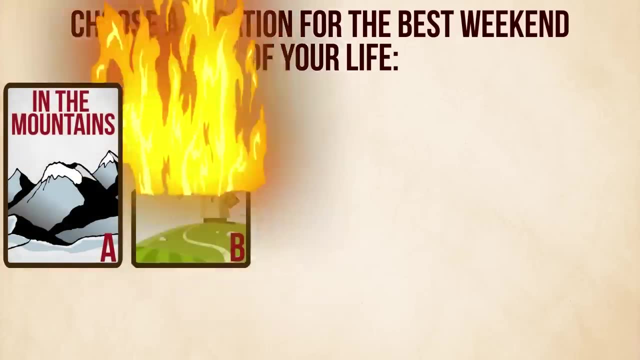 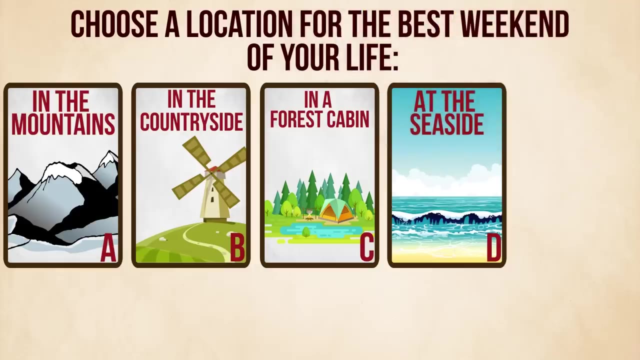 Question number 8.. Choose a location for the best weekend of your life: A In the mountains, B In the countryside, C In a forest cabin, D At the seaside. E Doing something extreme like rock climbing or abseiling. 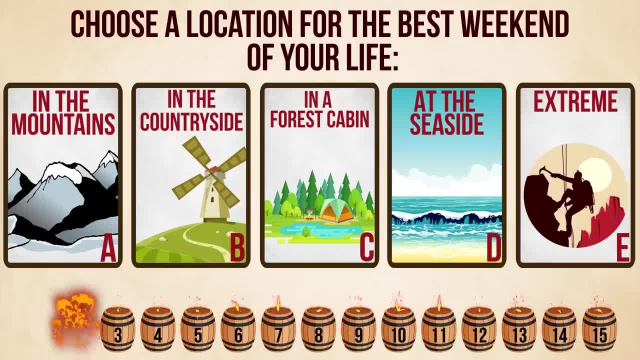 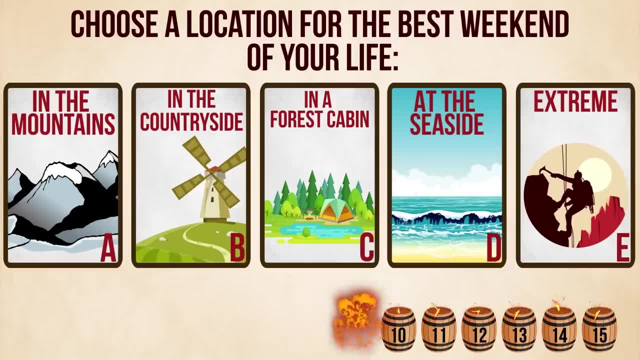 Question number 9.. Choose a place to go to: A To the beach B To the beach C To the beach D To the beach D To the beach C To the beach D To the beach. 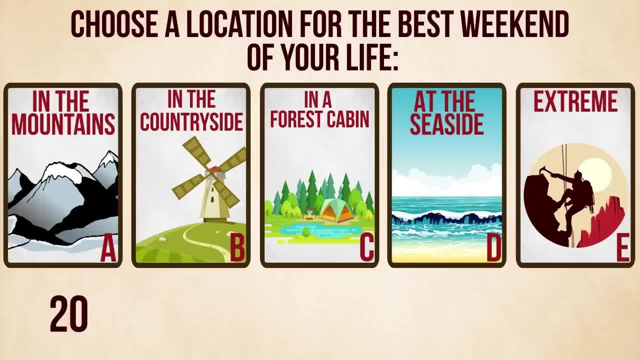 C To the beach. D To the beach. Question 7 came in first with 50 points and C is worth 40.. If you've opted for D, that's 10 points to your score. As for those who prefer thrill of answer E, you get 30 points. 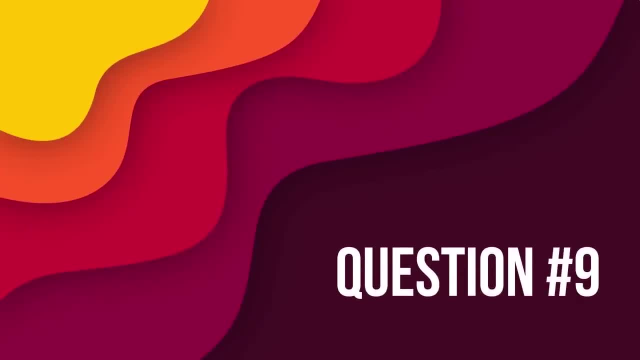 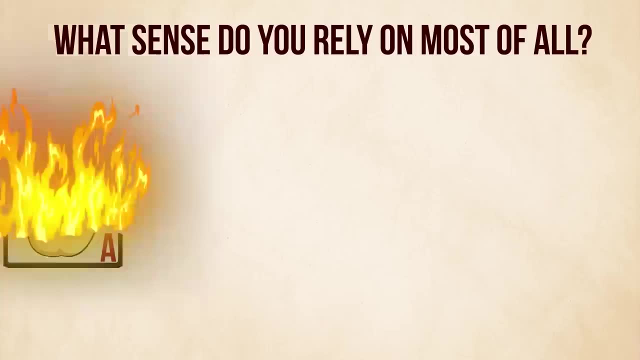 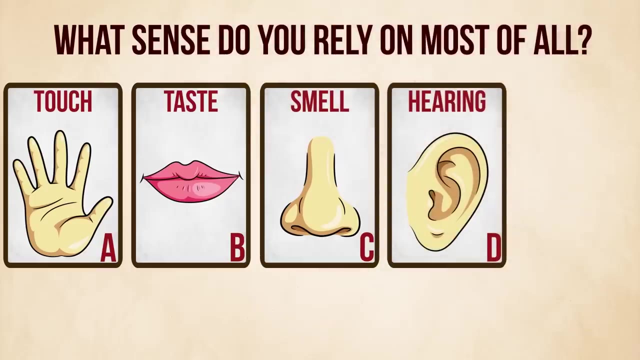 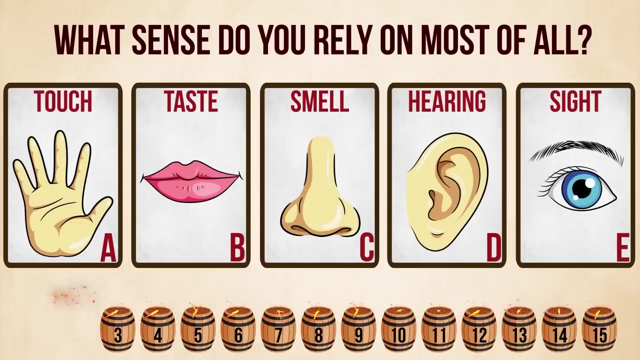 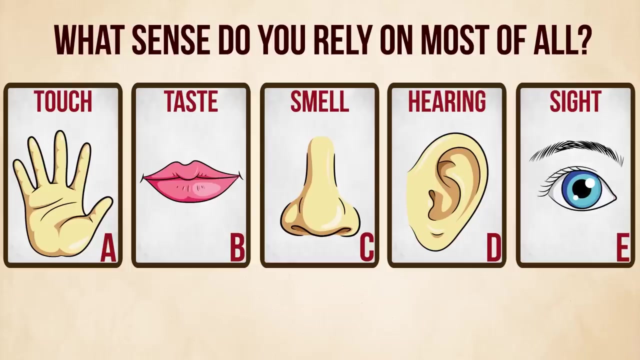 You said you knew the answer right. Correct Question number 9.. What sense do you rely on most of all? A Touch, B, Taste C, Smell D, Hearing, E, Sight, E, Sight Score. 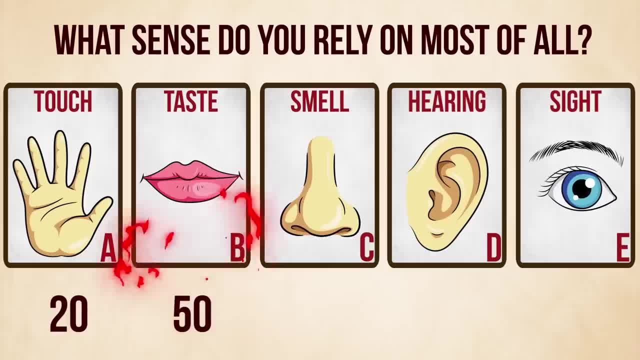 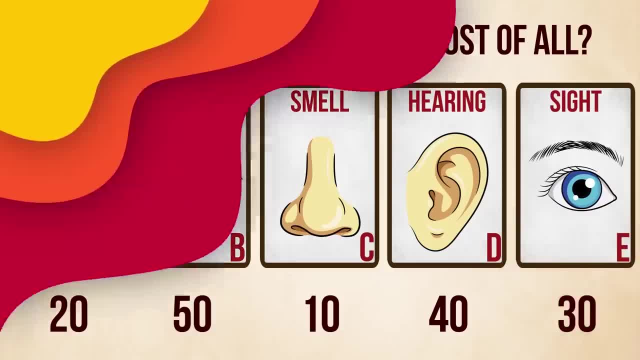 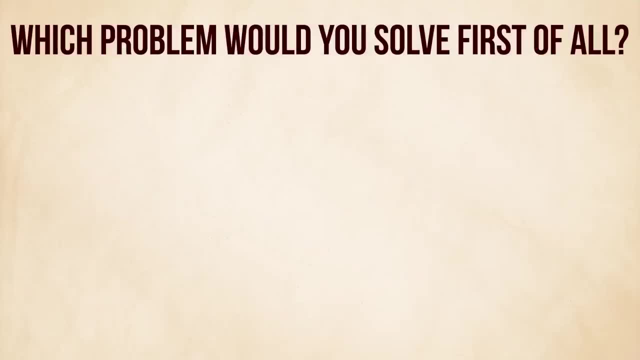 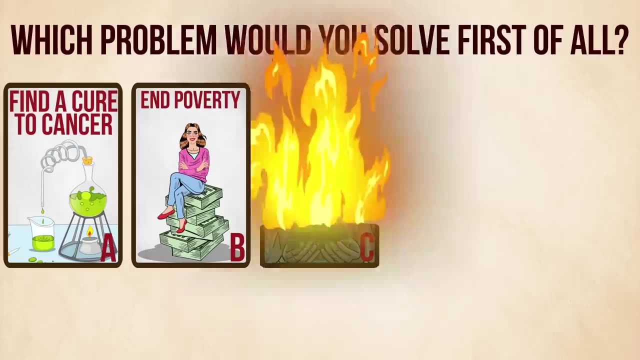 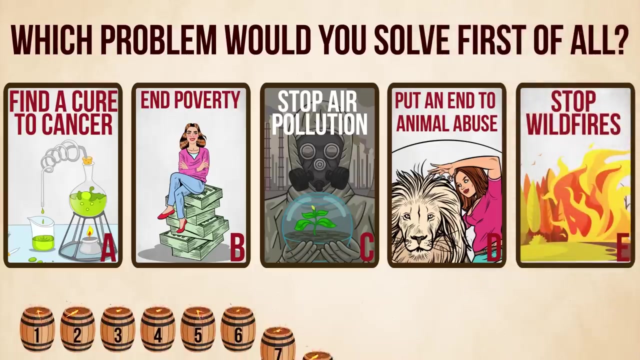 For choosing: A you get 20 points, B is 50 points, C is worth 10, D is 40 points and E gets you 30 points. Question number 10.. Which problem would you solve first of all? A- Find a cure to cancer. B- End poverty. C- Stop air pollution. D- Put an end to animal abuse. E- Stop wildfires. 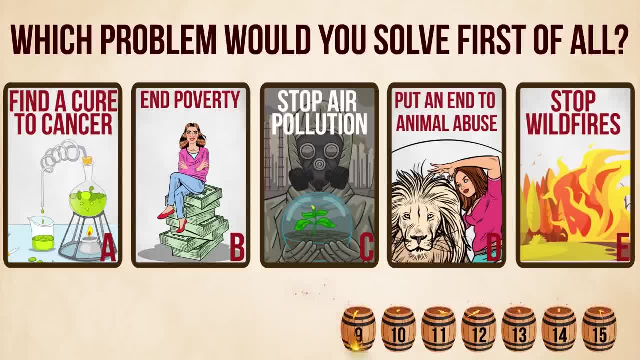 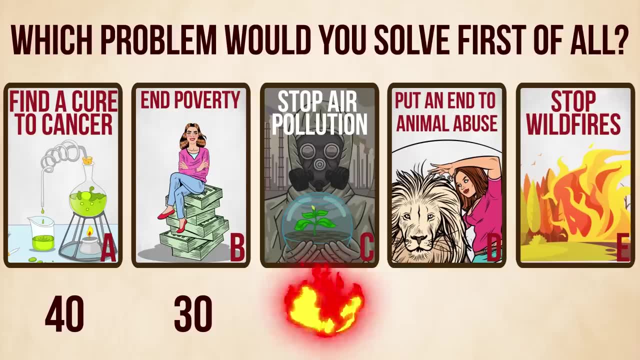 Question number 11.. Score: If you went for A, you get 40 points. B is worth 30 points. if C seems like the best answer, that's 20 points. D will give you 10 points and E is worth 50.. 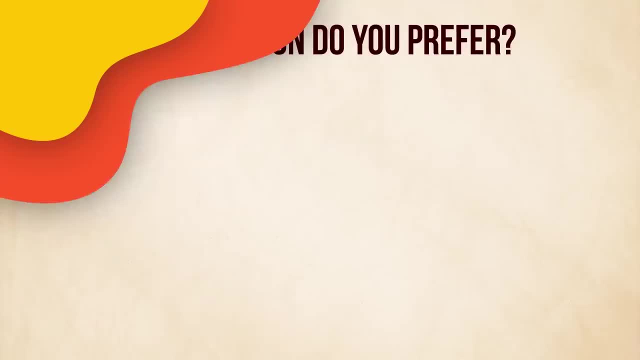 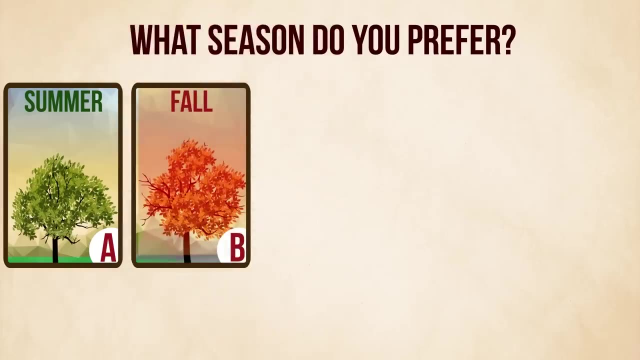 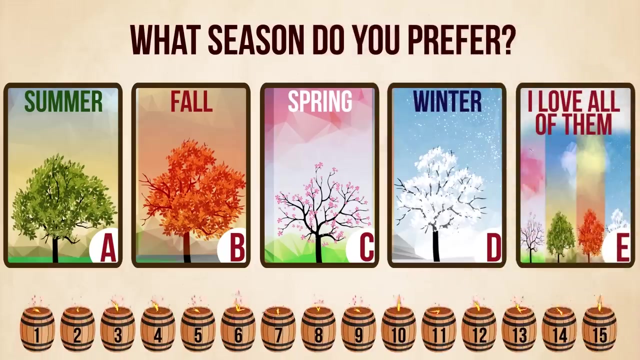 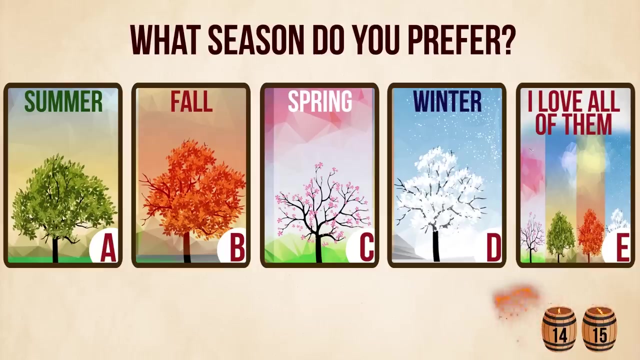 Question number 11.. What season do you prefer? A Summer B, Fall C, Spring D, Winter E. I love them all. Score. If you're a summer lover, you get 40 points for choosing A. 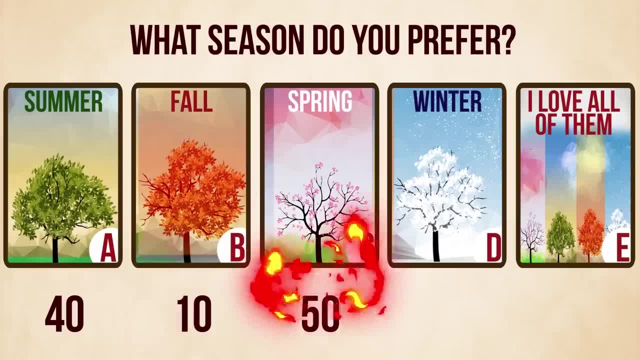 Answer: B will award you 10 points and C will give you 50.. Add 30 points to your tally. if you chose D, And if you just love them all and went for E, you get 20 points. Question number 12.. 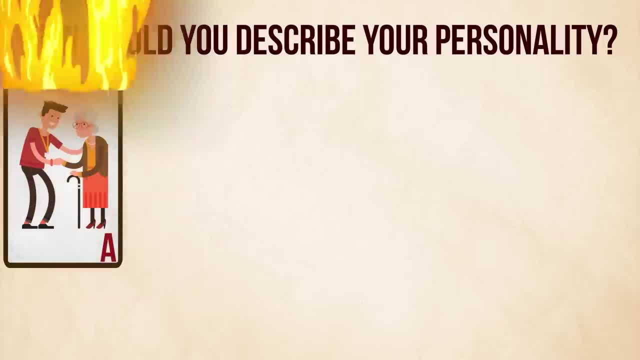 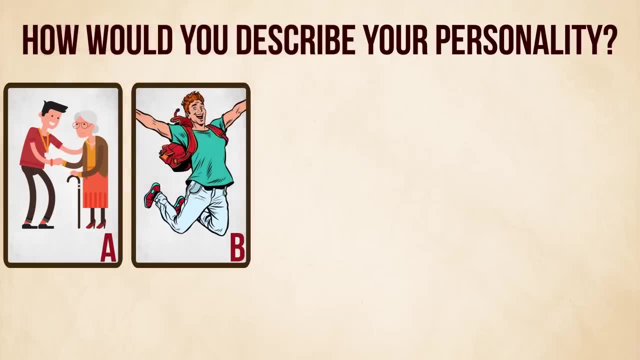 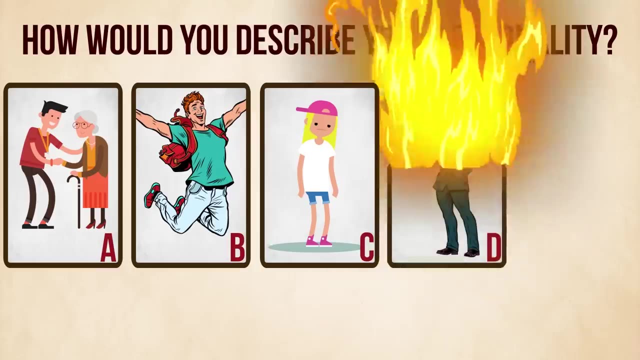 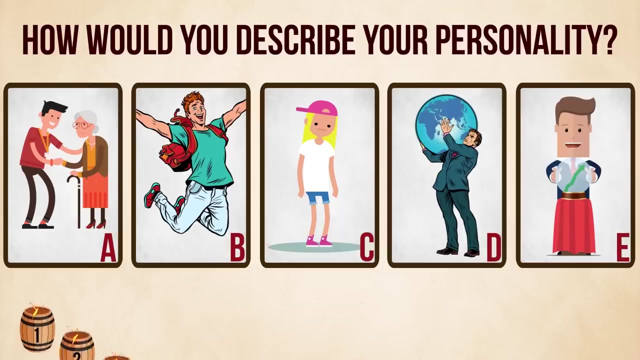 How would you describe your personality? A- I'm friendly and always try to do something for those who need help. B- I'm super energetic. I don't like staying in one place for too long. C- I'm a sensitive person. my surroundings influence me a lot. D- I love a challenging problem. it makes me feel good when I solve it. E- I'm good at analyzing things and predicting outcomes. 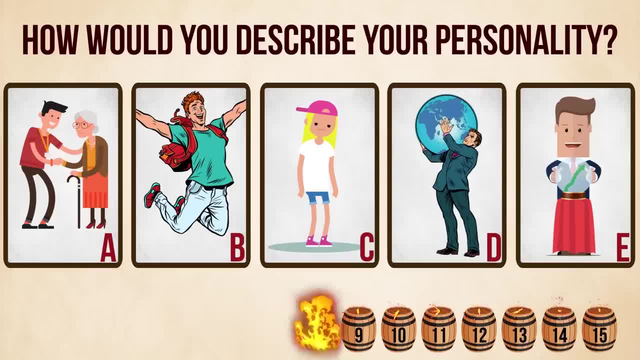 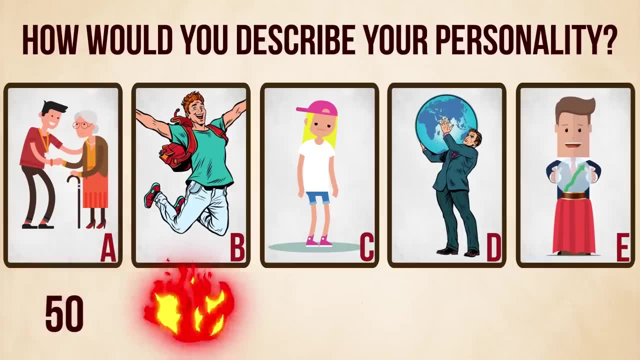 Answer B will award you 10 points and C will give you 30 points. and E. I'm good at analyzing things and predicting outcomes Score. If you like answer A the most, add 50 points to your score. Choosing B will give you 30 points and C is worth 10 points. 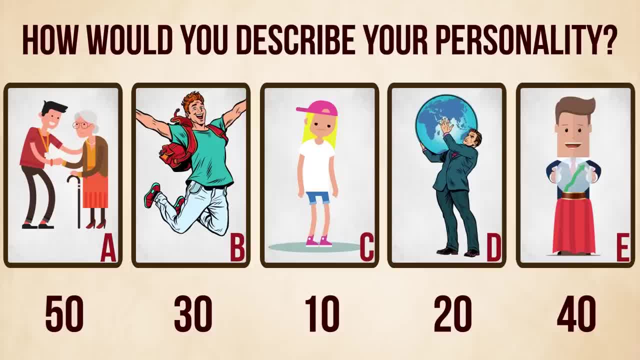 You get 20 points for D and 40 points for choosing E. Now it's time to add up your final score. You can always pause the video if you need a little more time with your questions. Are you ready? If so, here are the results. 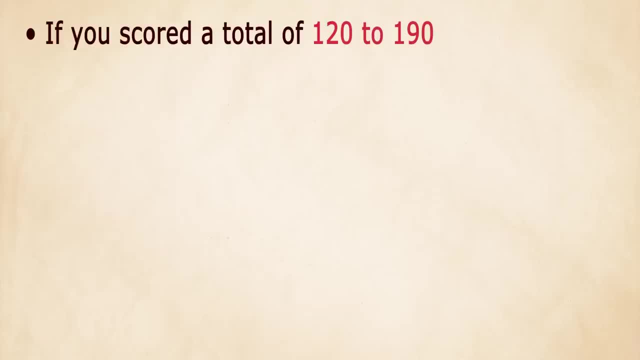 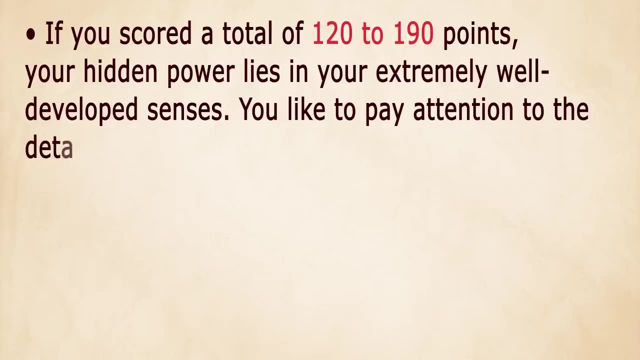 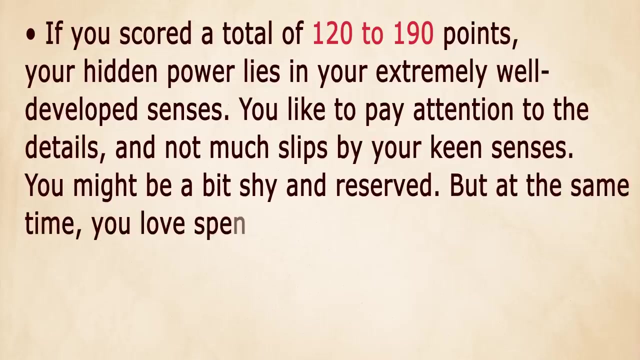 If you scored a total of 120 to 190 points. your hidden power lies in your extremely well-developed senses. You like to pay attention to the details and not much slips by your keen senses. You might be a bit shy and reserved, but at the same time you love spending time with your friends. 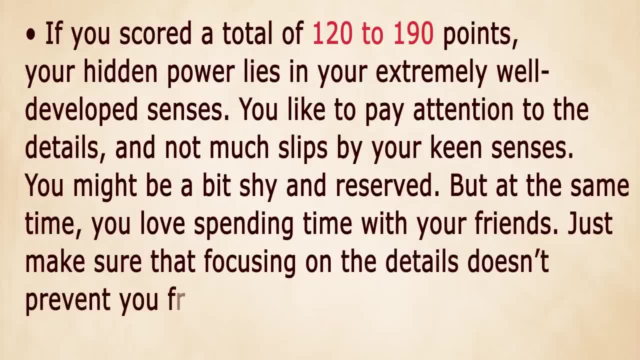 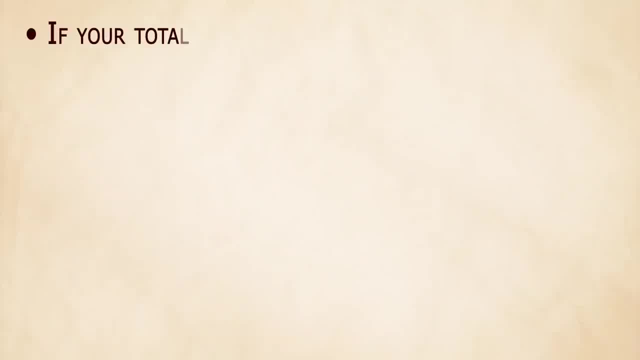 Just make sure you have a good time with your friends. Just make sure that focusing on the details doesn't prevent you from seeing the big picture. If your tally is between 200 and 290 points, your hidden power is your intelligence. And I'll tell you what. you're much more intelligent than you think. 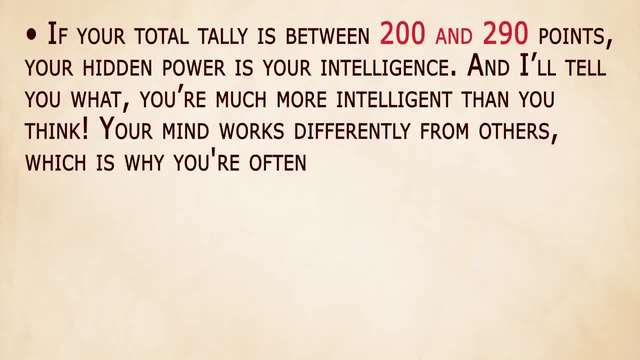 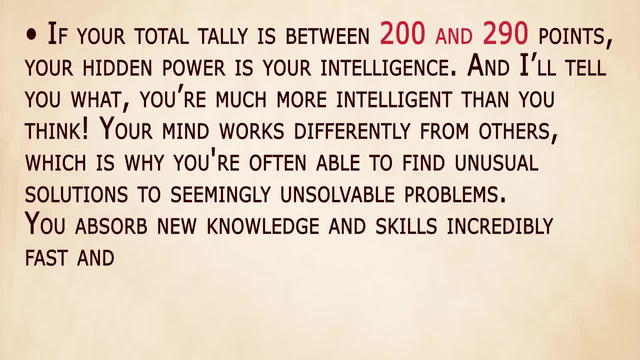 Your mind works differently from others, which is why you're often able to find unusual solutions to seemingly unsolvable problems. You absorb new knowledge and skills incredibly fast and are able to solve problems that are hard to solve. You're able to solve problems that are hard to solve. 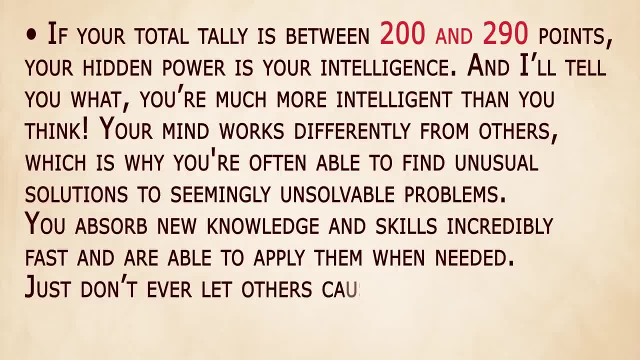 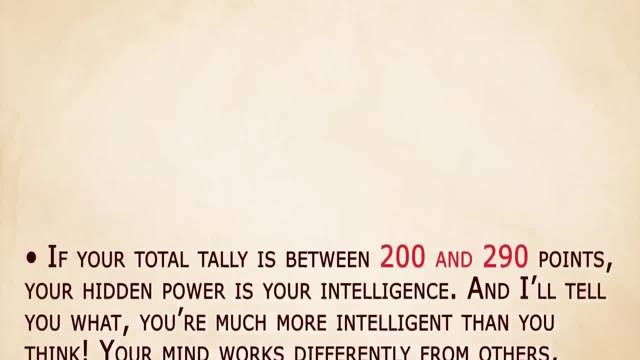 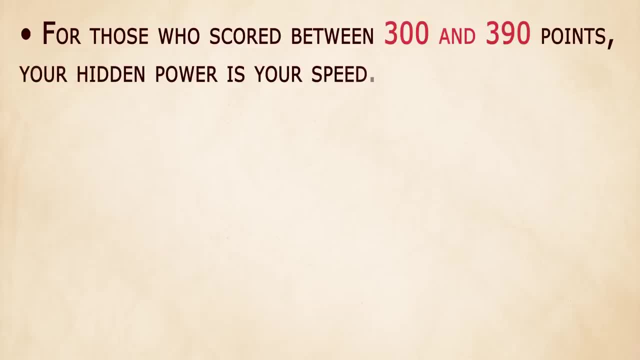 And you're able to apply them when needed. Just don't ever let others cause you to doubt or second-guess yourself. For those who scored between 300 and 390 points, your hidden power is your speed. You're rarely late and often arrive to meetings earlier than everyone else. 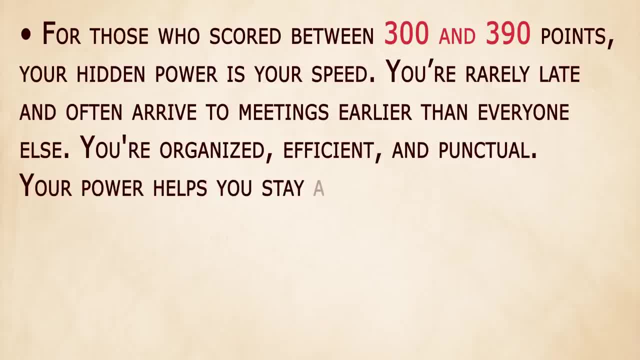 You are organized, efficient and punctual. Your power helps you stay ahead of time and manage to get much more done than most people can do. Your sense of timing improves as you might start to find and concentrate on something that's very, very difficult to achieve, though. 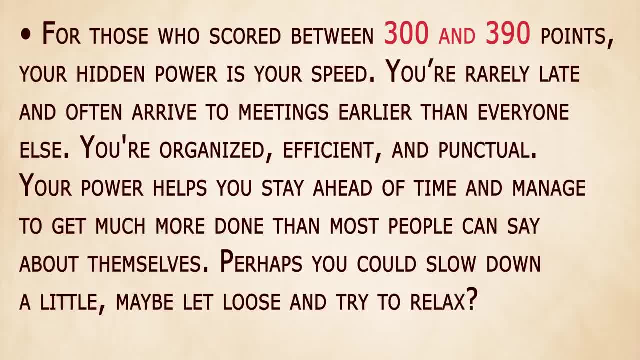 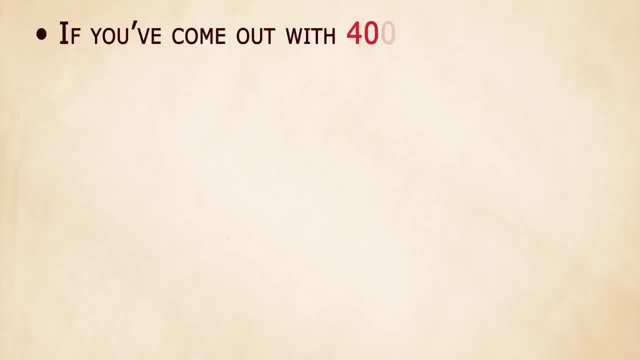 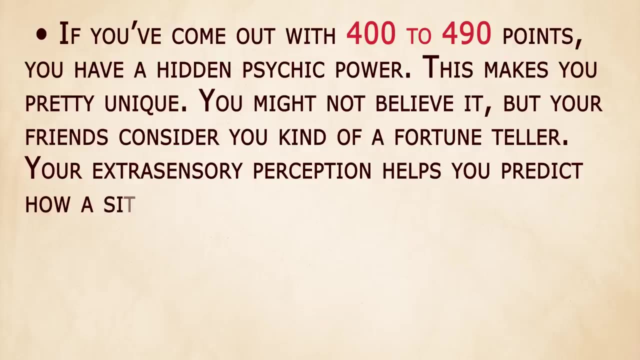 Perhaps you could slow down a little. maybe let loose and try to relax. Maybe let loose and try to relax. Absolutely not If you've come out with 400 to 490 points. you have a hidden psychic power. This makes you very unique. You might not believe it, but your friends consider you a kind of a fortune teller. Your extra sensory perception helps you predict how a situation will turn out or correctly guess what people are thinking about. 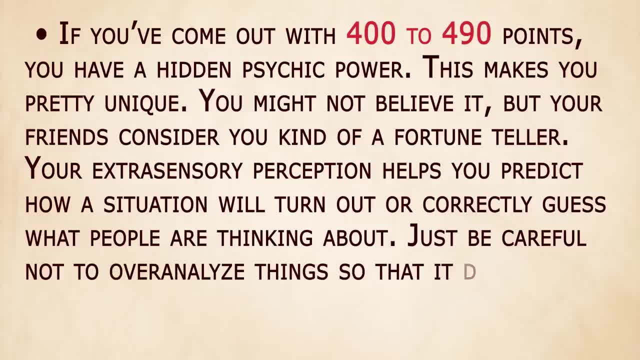 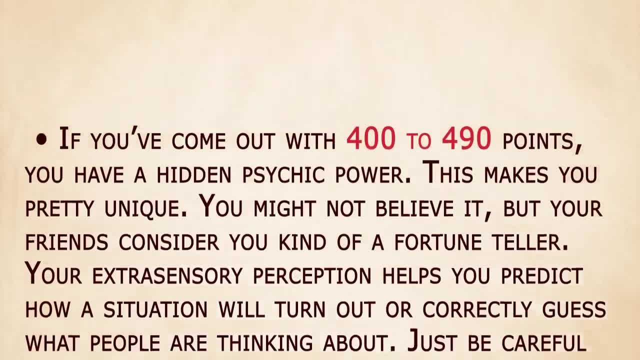 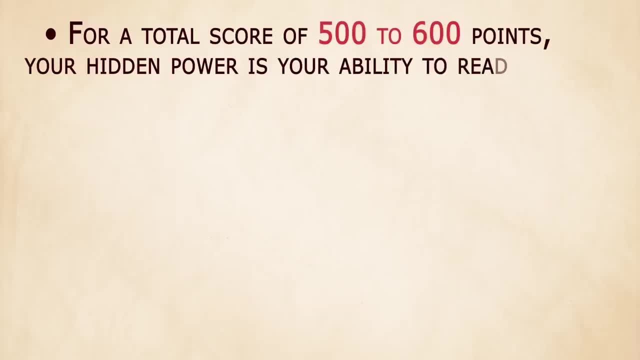 out. Just be careful not to overanalyze things so that it doesn't keep you from living your life today For a total score of 500 to 600 points. your hidden power is your ability to read people like a book. You can easily understand when somebody is lying and you know when people 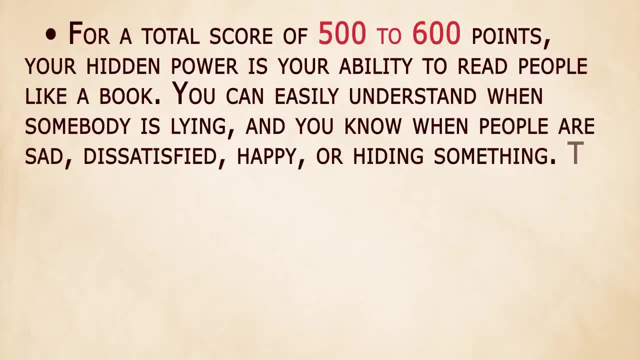 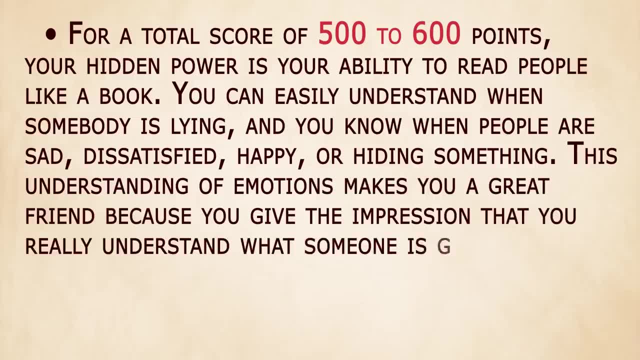 are sad, dissatisfied, happy or hiding something. This understanding of emotions makes you a great friend, because you give the impression that you really understand what someone is going through. However, you're also great at concealing your own emotions from others. 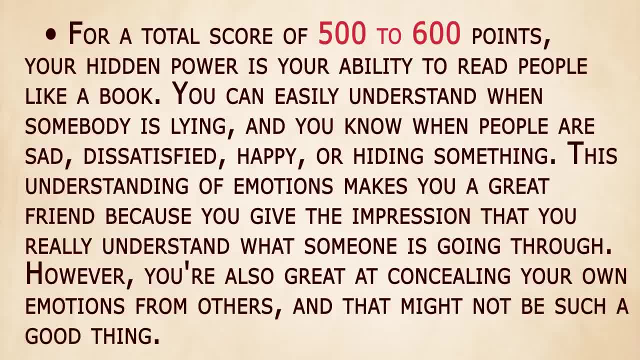 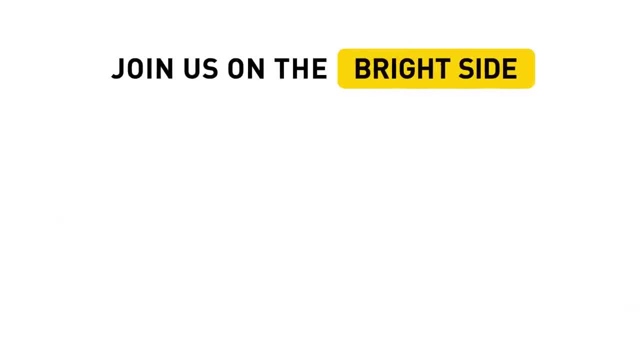 and that might not be such a good thing. What is your hidden power according to this test? Do you think it's true about you? Tell us in the comments below. Remember to hit the like button and always stay on the bright side of life. you.